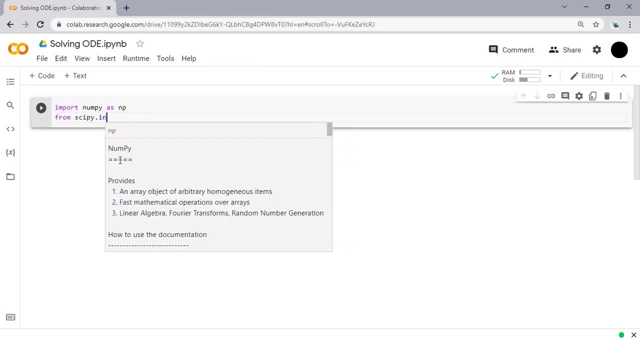 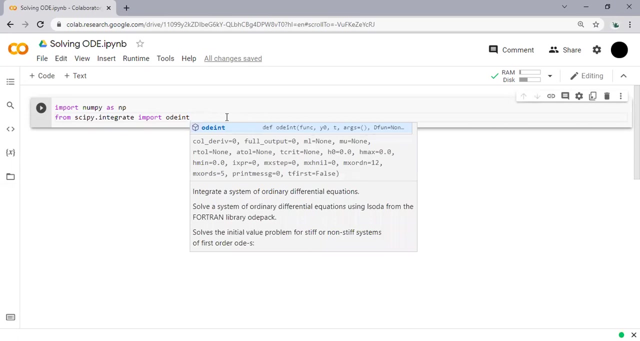 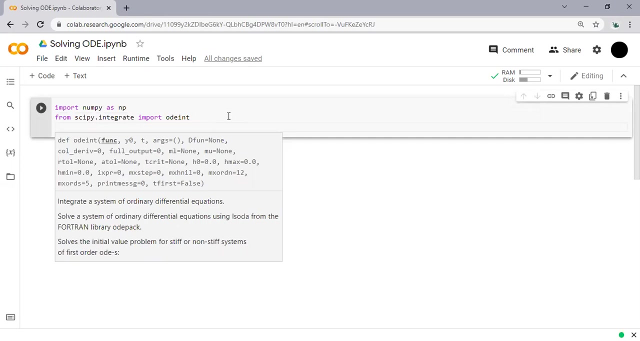 scipy integrate, because solving ode or differential equation, it means integrating the differential equation and then we will use scipy to integrate the differential equation right to get the solution. so from scipy integrate we will import the ode int, ode int, integrating the ode right and the second or the third one. i will use matplotlib in order to be able to plot all. 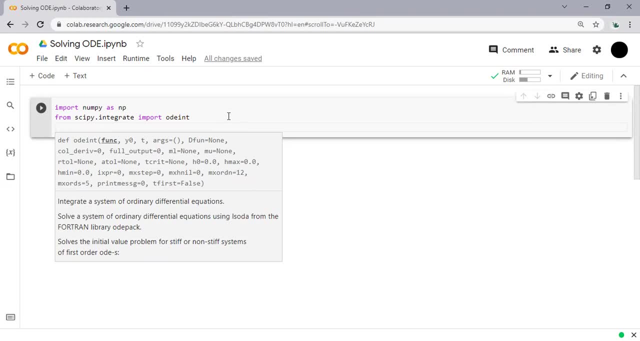 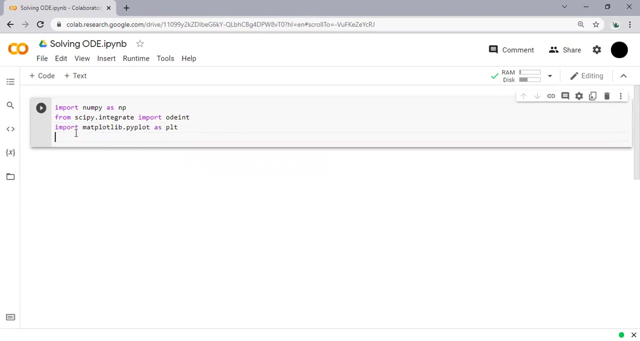 right. so if you get the solution, you plot the solution and that's it. so we will use matplotlib, import matplotlib, this one, and we will use the pi plot. so import the matplotlib dot pi plot and we call it splt, and then we divine the equation. divine equation, it has two arguments: time and y. 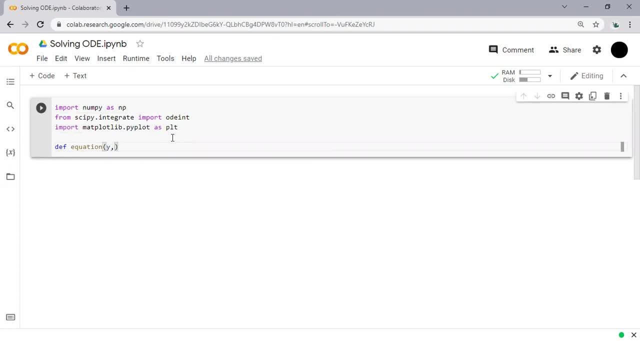 the first one is y, the parameter, and the second one is time, or we call it st alright, and then colon, and then the ode itself, d y d t, differential of y with respect to time. and let's say: this is the function five times y minus three. that's our equation, and then we will return d y d t. okay. we will call back the dy dt and we are going to return d y dt. yes, right. and when we go back let's said that the spicy Ft to be a using Esther and our parameters are not there yet so we can find out what's written down there at rest of the alright and then colon and slash these two factors. 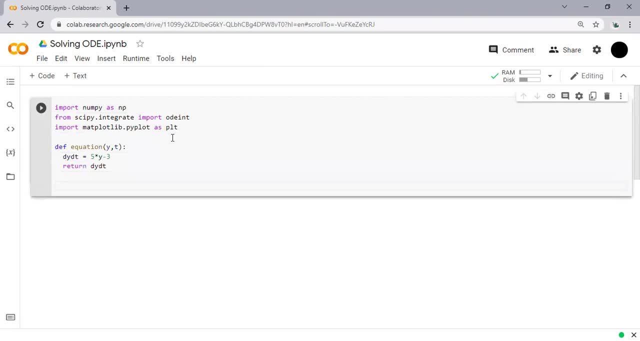 write the prótico combination to try to define the operative stringשה. And then, for example, we have the initial solution, Y0. We call it Y0 and the Y0 is 10, for example. So we divide, Y0 equals to 10.. 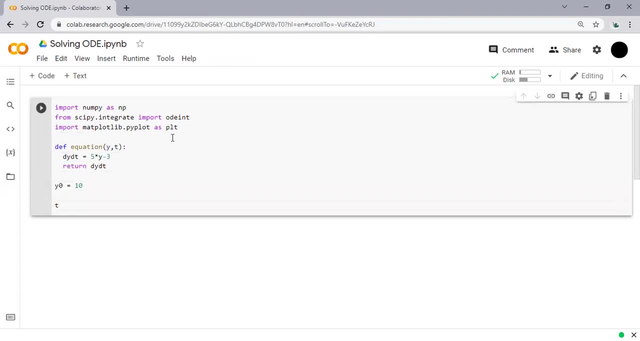 And then we need to describe the time. T. we call it T equals. Now we will use numpy to create linspace. numpy dot linspace, For example, the time will be from 0 to 5.. Okay, so that's it. 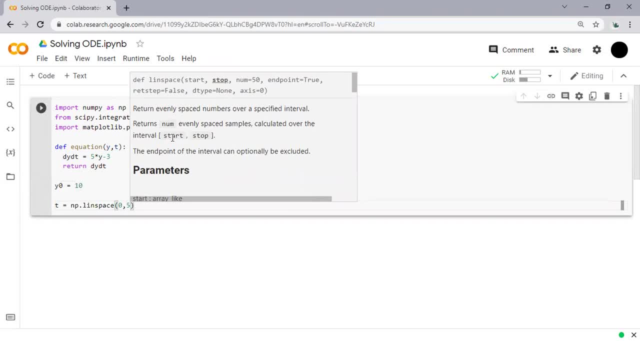 Np, dot, linspace, right, And it will give us linear space range from 0 to 5. Maybe, like, if there will be 10 points, So 0 comma, something comma, something as much as 10 until 5.. Okay, But we can't. 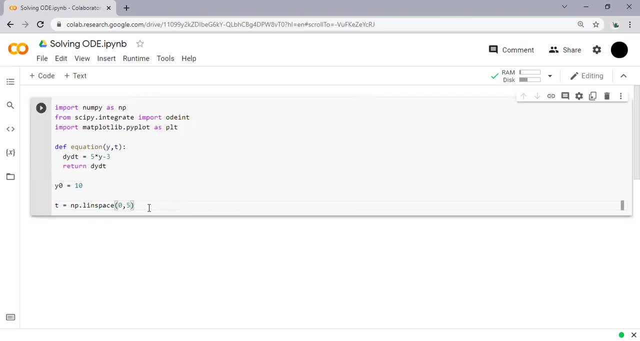 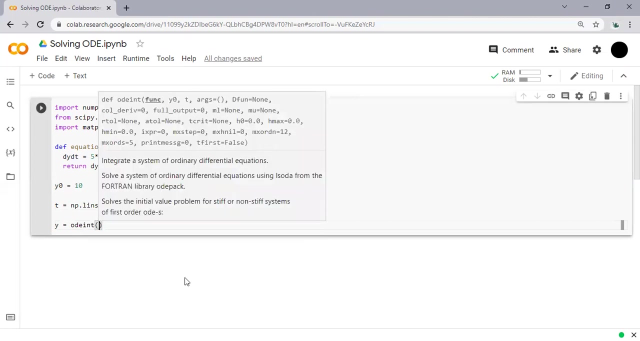 We can skip that. We only have 0 to 5.. And then the solution Y. We can get the solution by using odint, odeint. This is the syntax. The first one is the function, And the function is equation defined here. 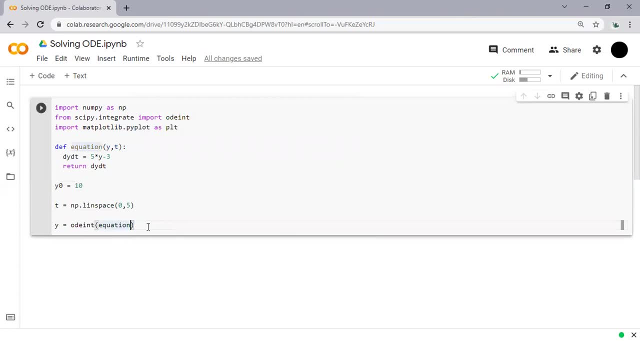 All right Here. equation. And then The second argument is the initial solution, which is Y0.. This one, All right. And then the third argument is time? All right, This one T. Okay, that's it for the solution generation. 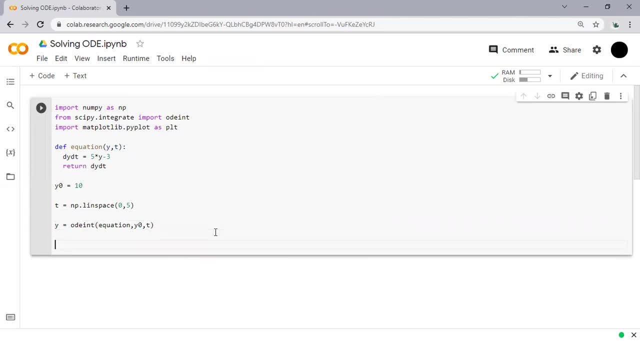 And the next one is to do the plotting: PLT, dot. plot T, comma Y. So the horizontal axis will be time and the vertical axis will be the solution or the Y, All right, And then we give the label PLT, dot, X label for the X axis. 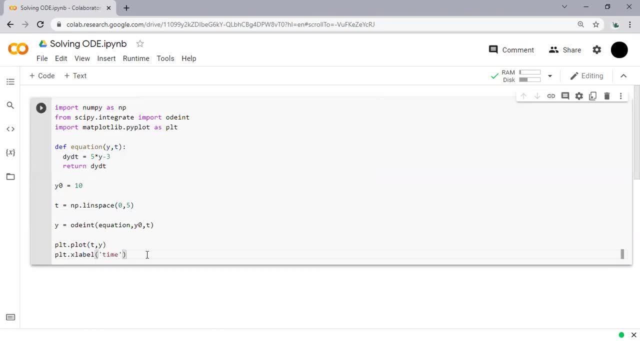 We call it time, And for the Y label, we call it Y- Okay. And then, lastly, we will show the plot. PLT dot show like this: Okay. And then maybe you want to know the T, We can also show T like this: 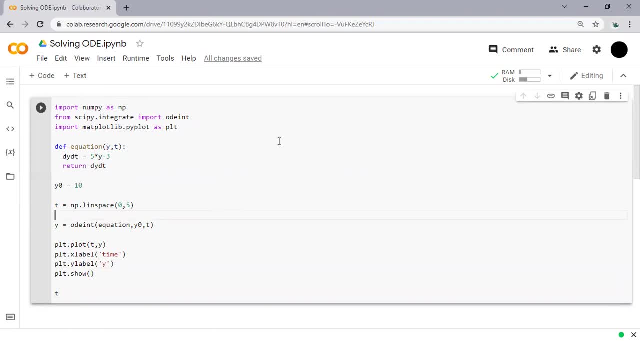 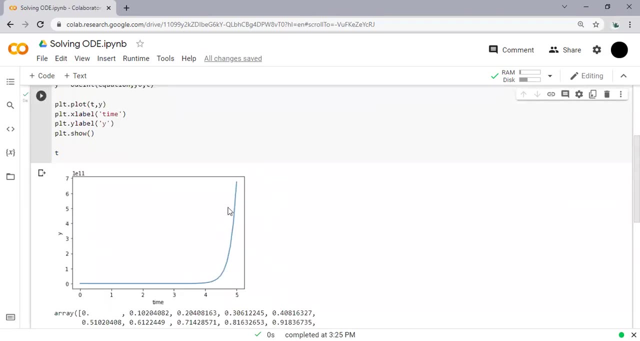 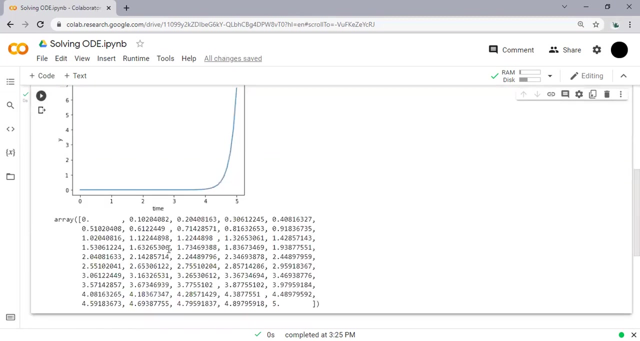 Okay, So so far, so good. We can run the code All right. So this is the solution. Y versus time. This is the plot. Okay, All right, And then this is the T, from zero to five. You can count one, two, three, four, five.